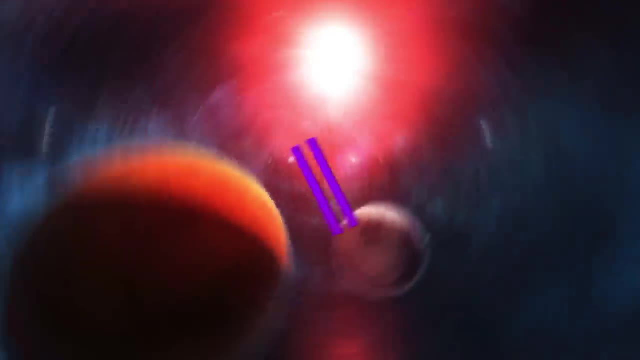 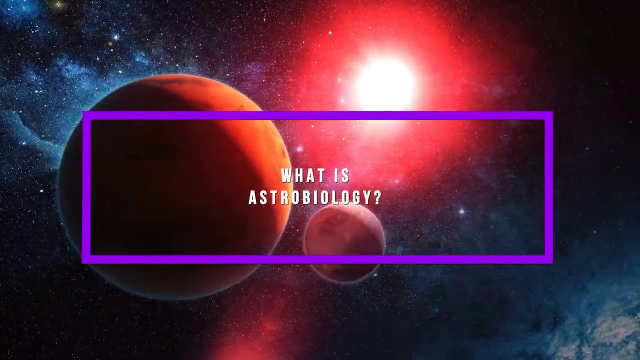 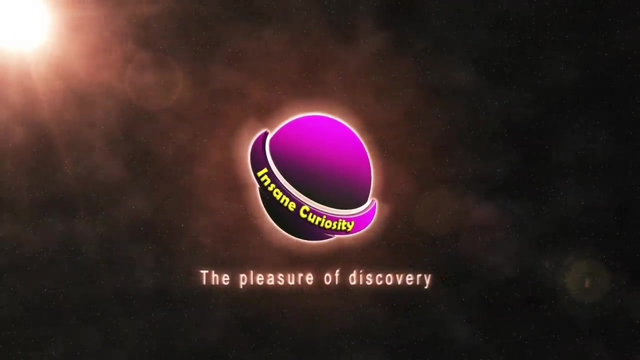 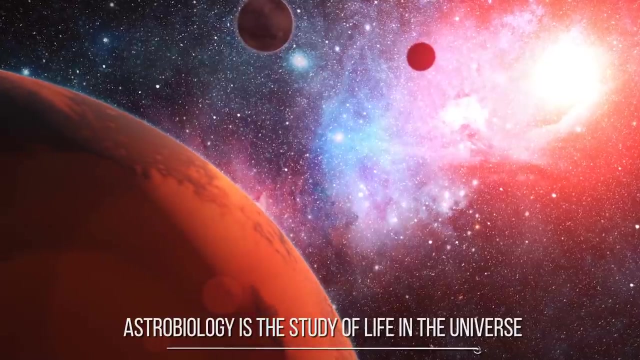 Astrobiologists try to answer this type of question. But what is exactly astrobiology? Follow me to get to know more about it. You won't regret it. Let's start by simply answering the question: What is astrobiology? As it's easy to imagine, 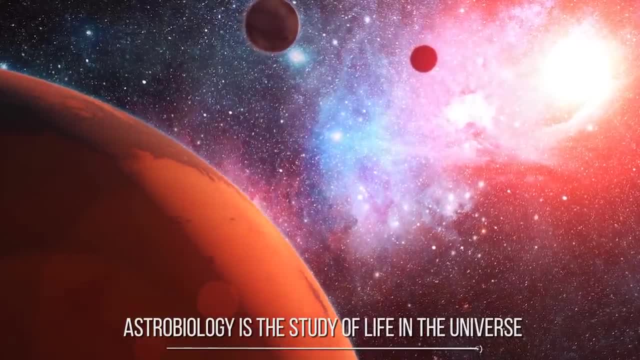 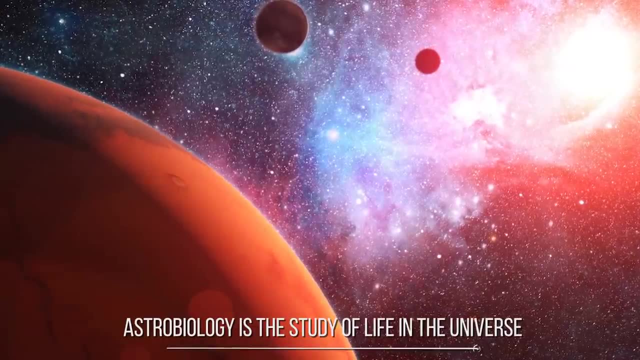 astrobiology is the study of life in the universe. Do you think it is an easy task? Well, I'm sorry to disappoint you, but life in the universe is actually one of the hardest things we can study. But let's go back for a moment. when the term astrobiology was invented, It was only in 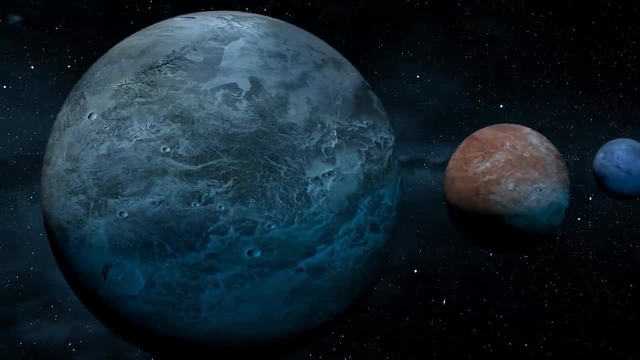 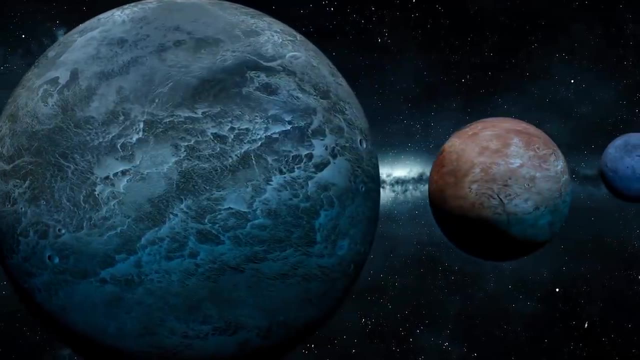 the 1950 space age that the term astrobiology was coined. It was used to define the study of the biological impact of space missions on dalli. The term astrobiology was also used to describe and to define the study of the search for extraterrestrial life. 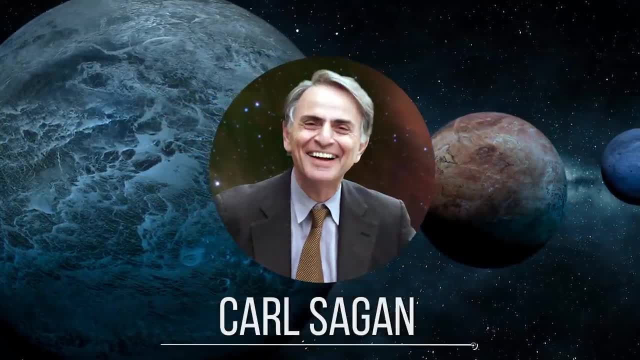 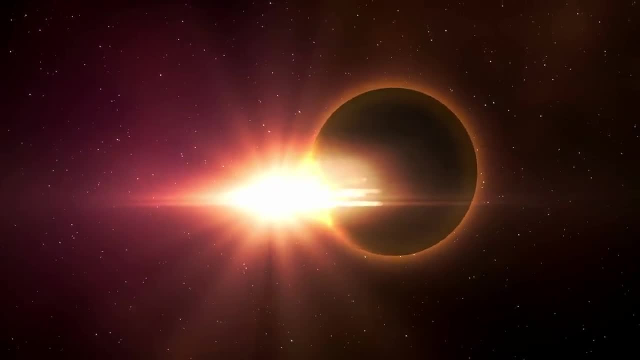 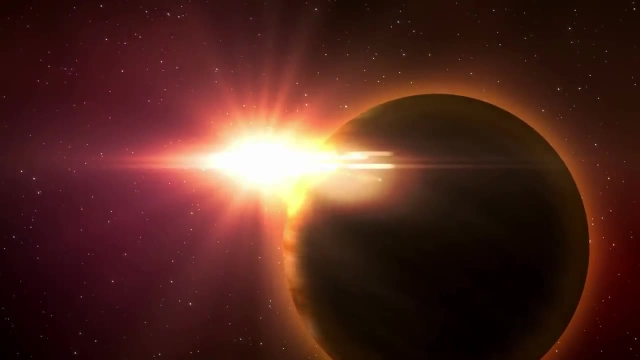 Later, famous scientist Carl Sagan brought astrobiology to the public and to the scientific community, and the field began to gain recognition. So nowadays, astrobiology is defined as the science that studies the origin, distribution and evolution of life in the universe, and it takes several branches of science. 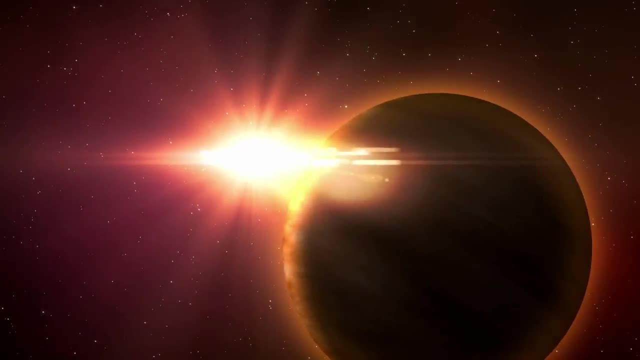 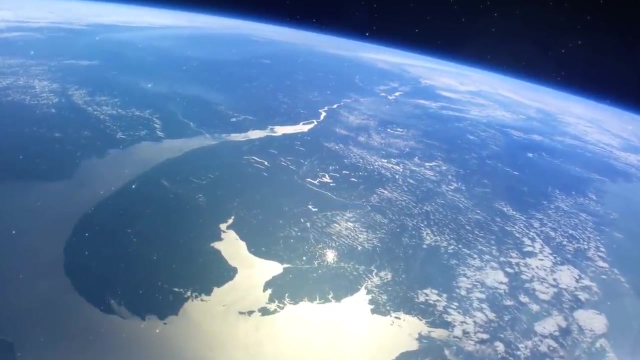 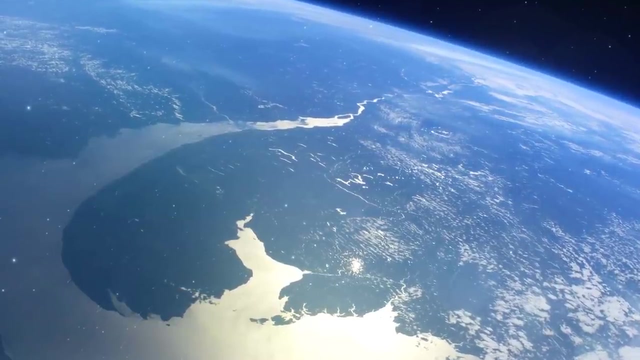 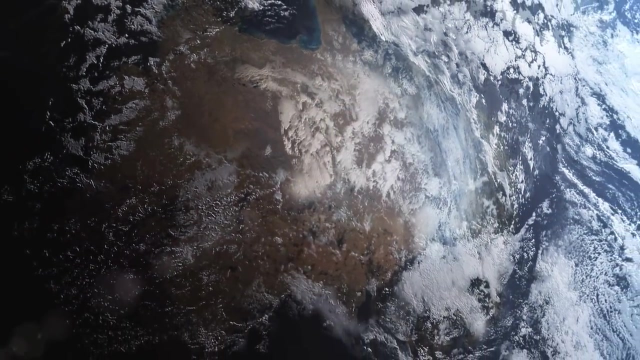 but also engineering and society, and brings them all together. Astrobiologists can work alone on particular scientific questions, but often astrobiologists from different scientific disciplines work together to examine complex questions that no one field can answer alone. When we think about life in other worlds, what we immediately start to imagine is little green men. 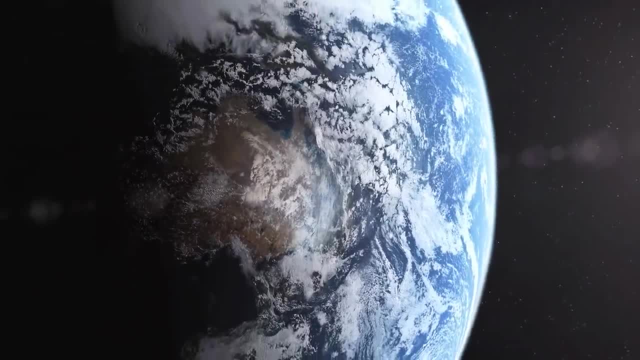 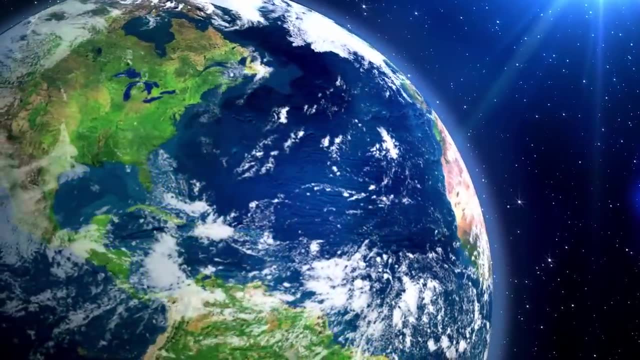 or maybe tall, intelligent species that invade our home Earth on their technologically advanced spaceships. but this is science fiction. Do you want to know what we really know about life in the universe? Let us know in the comments. Well, if we want to speculate about life in other worlds, what could it be? 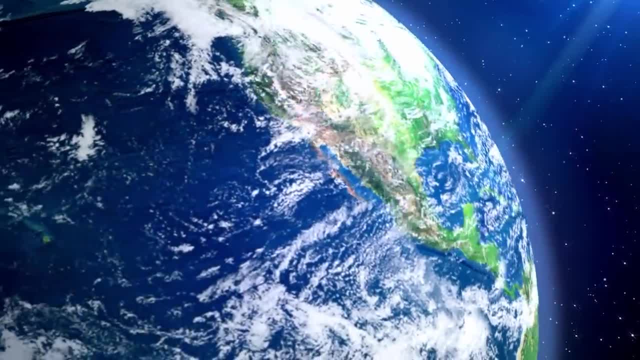 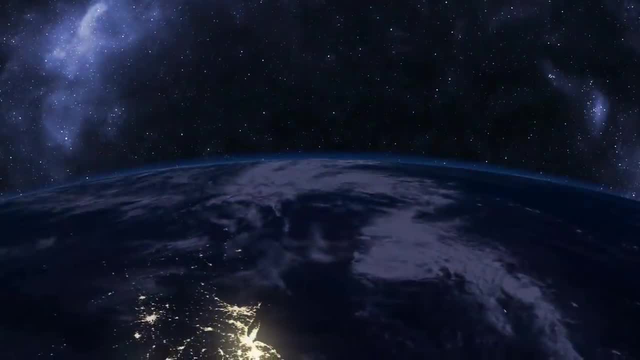 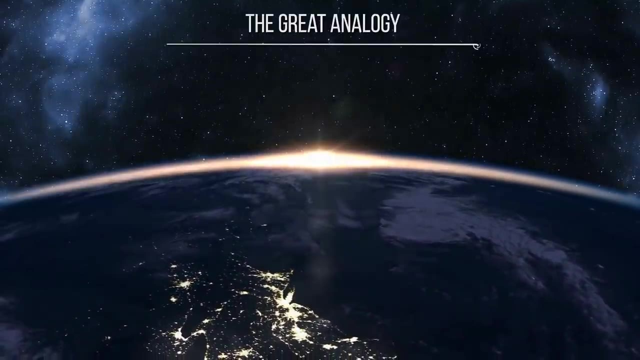 One of the logical starting points, and maybe the only one, is to start by looking at our own planet. In fact, for now, the only known planet hosting life is Earth. You'd say this is pretty obvious, right? So what do astrobiologists do next? They use a method called the Great Analogy, In short. 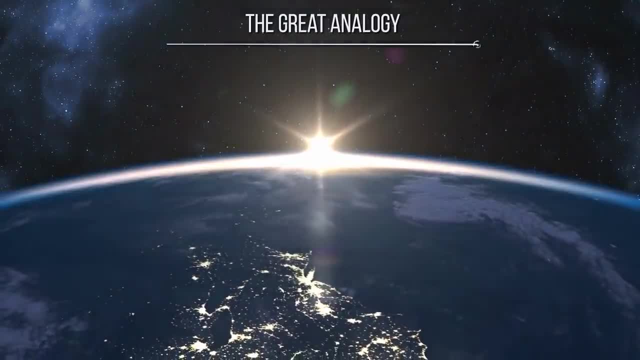 terms. they use the knowledge that they have from life on Earth, how it originated and evolved. Then they try to figure out the origin of life on Earth and how it evolved. Then they try to understand how to extrapolate that knowledge to other environments in the universe. 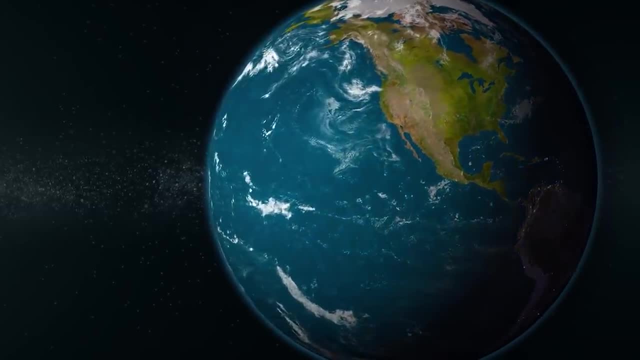 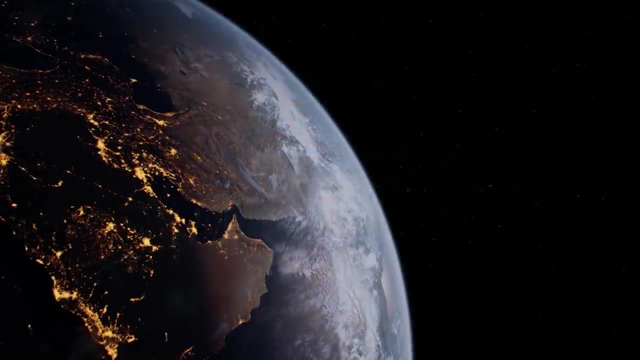 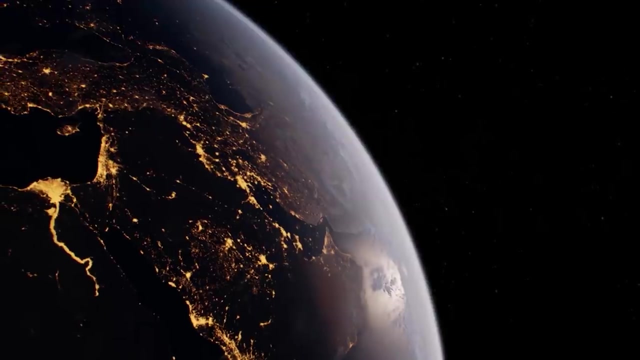 such as our solar system. That's why the understanding of the origin of life on Earth is the main key in order to give a push to astrobiology. The question now is: what do we know about life on Earth? We know that here on Earth, life emerged around 3.8 billion years ago. 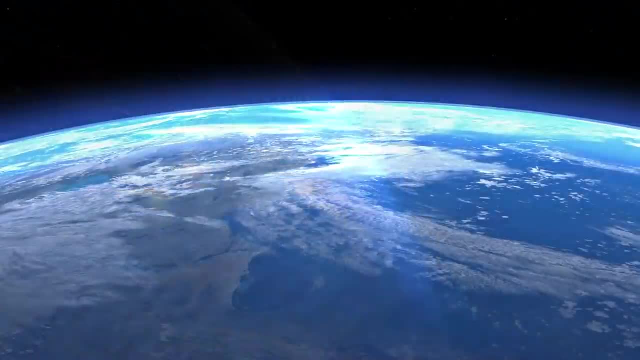 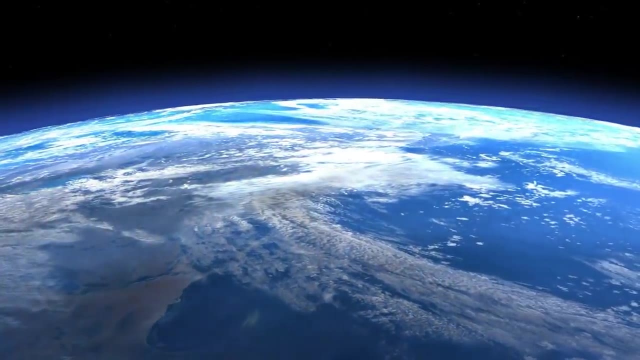 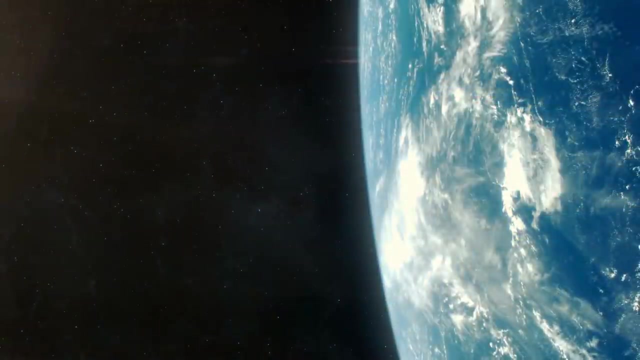 probably in the deep oceans. Why? Well, we know that back then, the Earth was not the same as today. What do we mean? We mean that if you were here, you could have not been able to breathe because there was no oxygen at all and there was no ozone layer. This means that we had a lot. 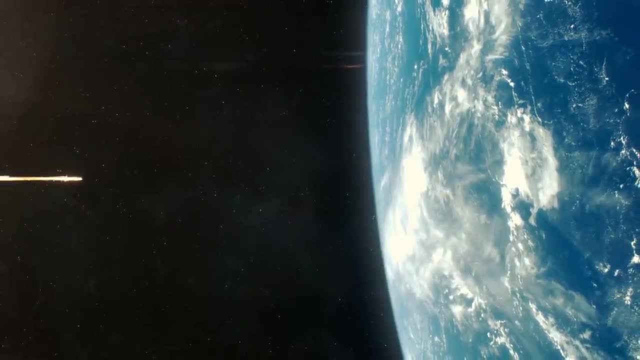 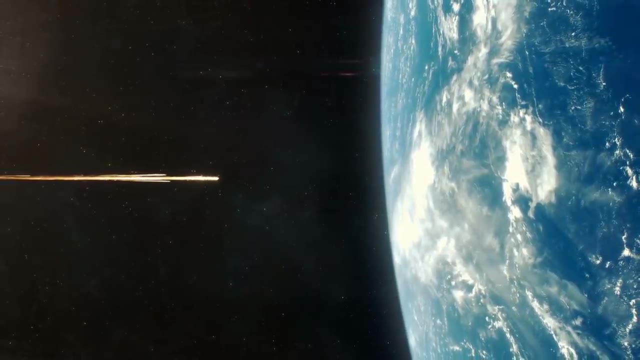 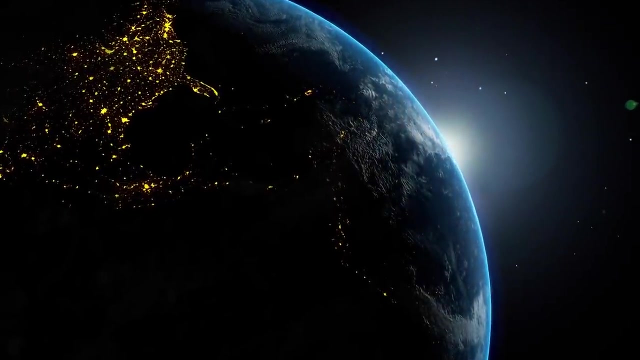 of radiation, and it brings us to the conclusion that the first forms of life would have to be anaerobic. They would have to avoid radiation and grow up without oxygen. That's why we think it originated in deep oceans. There, the radiation isn't an issue. These are our first clues about. what it takes for life to evolve. If you want to know more about life on Earth, subscribe to our channel and let us know what you think about life on Earth. If you want to know more about life on Earth, subscribe to our channel and let us know what you think about life on Earth. 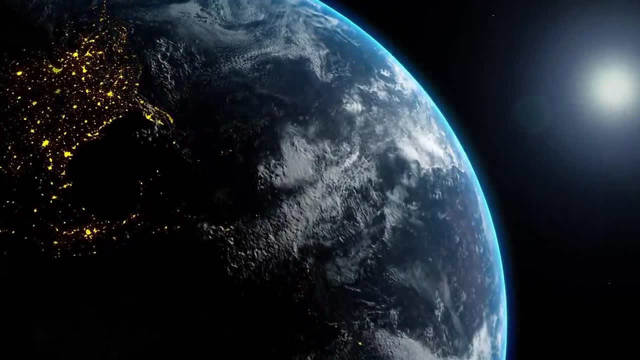 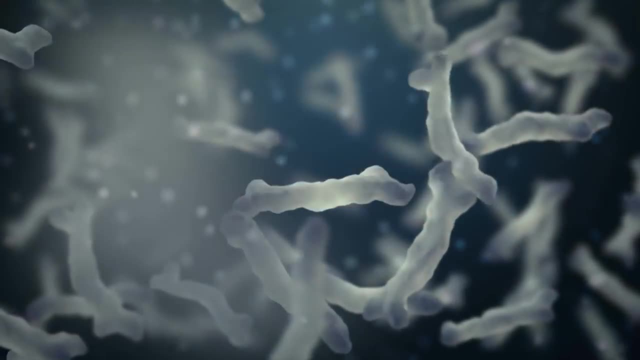 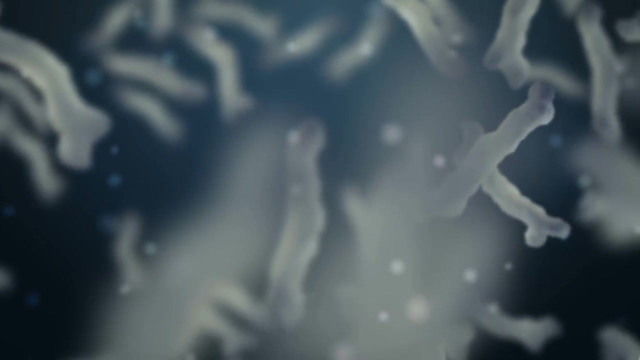 Liquid water and organic molecules. What we think is that the oceans brought the molecules around and eventually the right molecules met at the right time and at the right place. That's how astrobiologists think life emerged. Also, by looking at the different life forms we study every day, we realize that 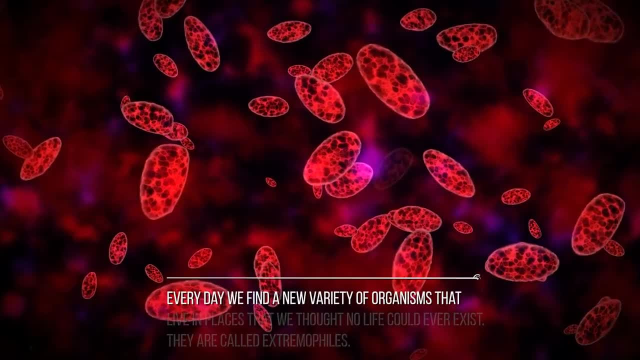 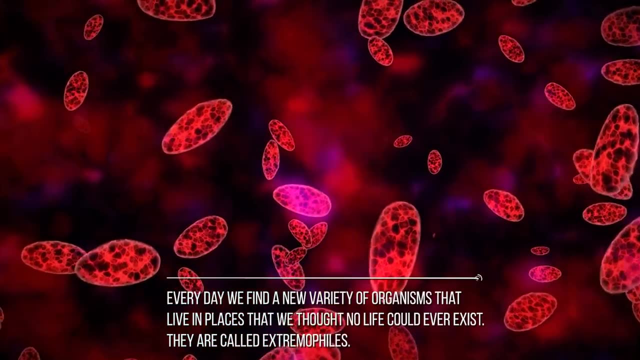 biodiversity is amazingly big. Every day we find a new variety of organisms that live in places that we thought no life could ever exist. They are called extremophiles. An extremophile from Latin extremis, meaning extreme, and Greek philia, meaning love. 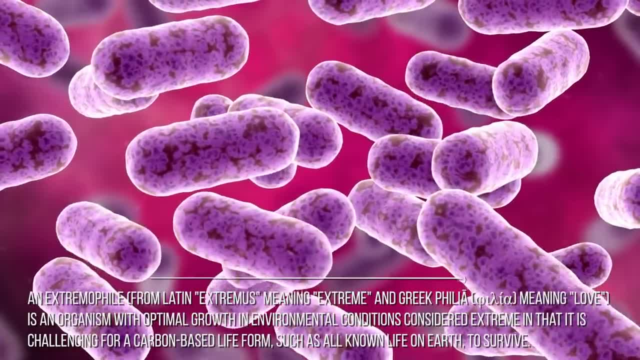 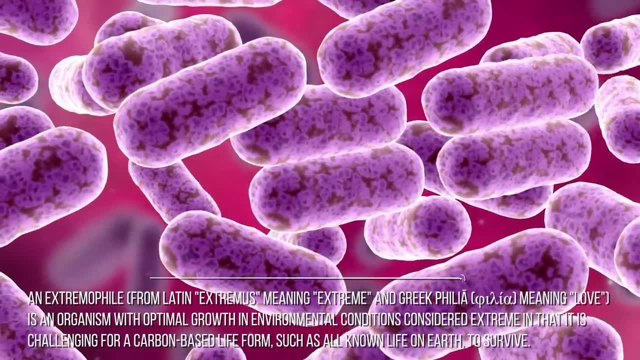 is an organism with optimal growth and environmental conditions, considered extreme in that it is challenging for a carbon-based life form, such as all known life on Earth, to survive. These organisms are dominants in the evolutionary history of the planet Dating back to more than 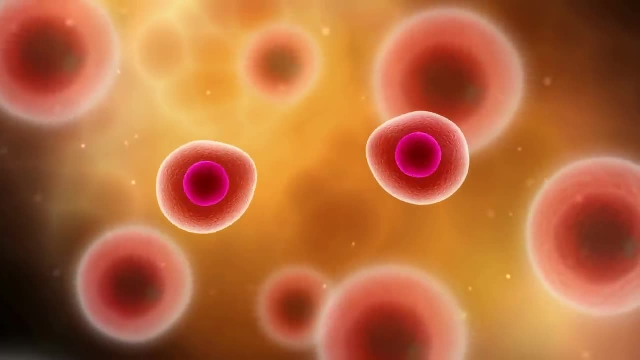 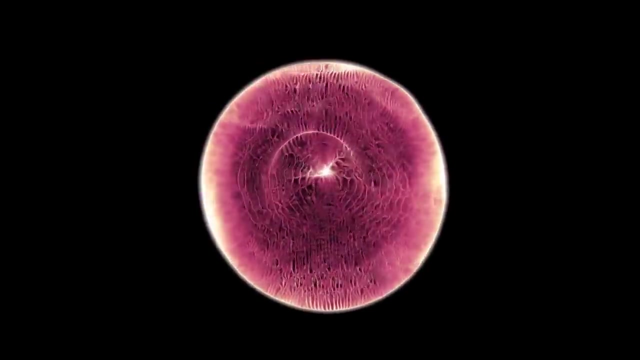 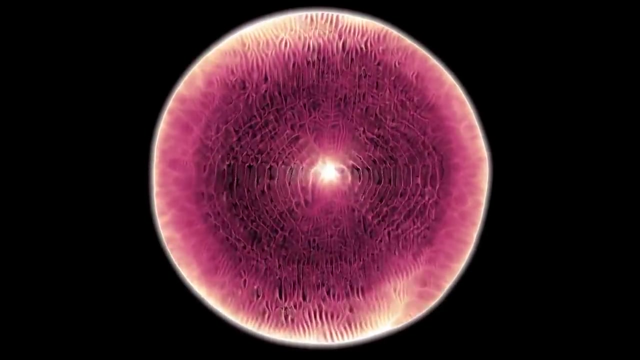 40 million years ago. extremophiles have continued to thrive in the most extreme conditions, making them one of the most abundant life forms. These microorganisms can live at temperatures above 100 degrees Celsius. Also, they live in acid rivers or very salty lakes, and they help us. 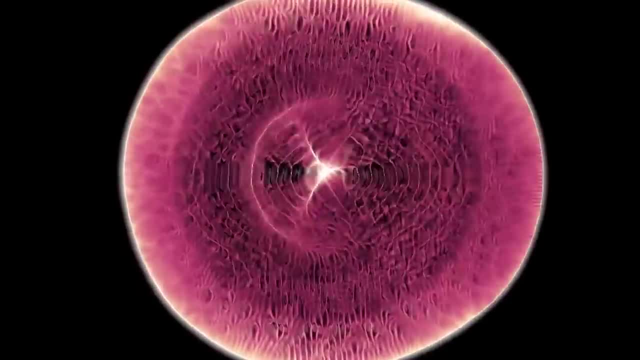 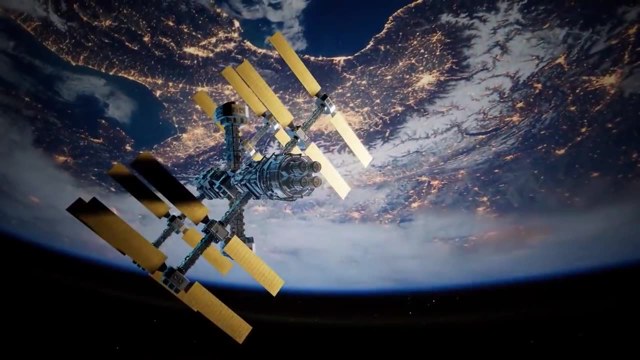 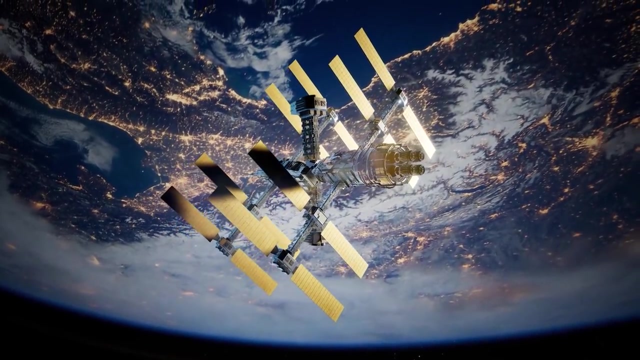 set the limits of life, Since one of the most extreme environments is actually space, astrobiologists ask themselves: can life survive in space? That's why they have done a lot of experiments in situ. They actually have sent bacteria and other microorganisms to space, put them on the 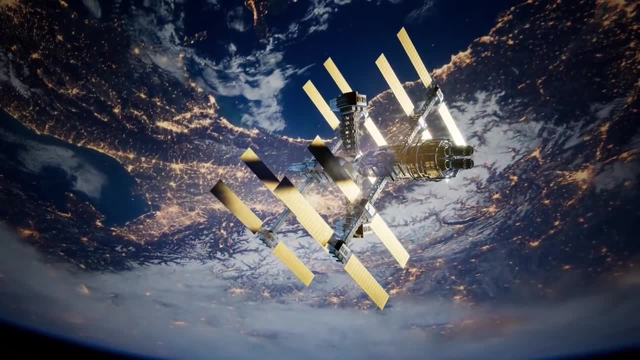 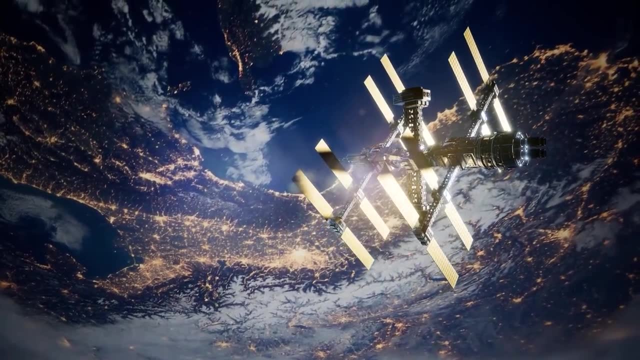 outside of the International Space Station, where they are exposed to the real space vacuum and the real space radiation. So they stood there for months and what they found is that many of them actually survived. This is a sort of a revelation, because it makes us wonder where. 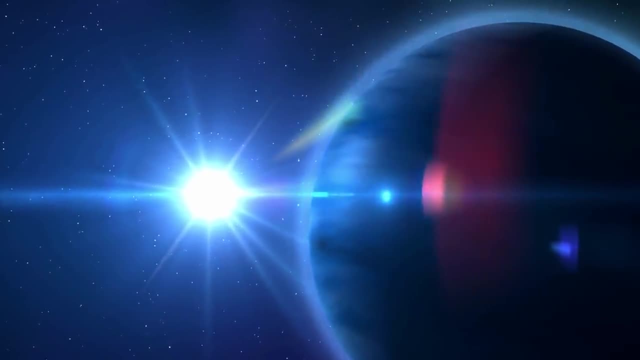 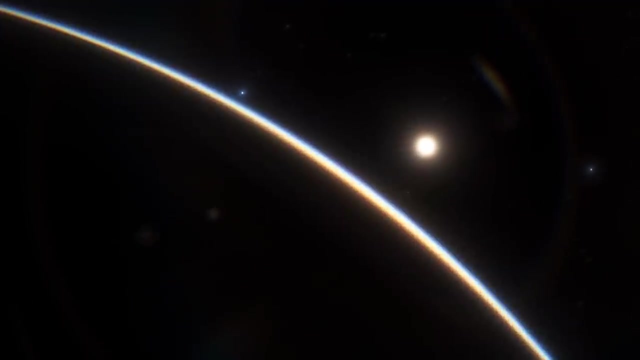 else in the universe can life survive. So the first place we actually look, of course, is our own solar system. We begin by looking at the moon. We went there. there is no life there, but then we focus on other things. 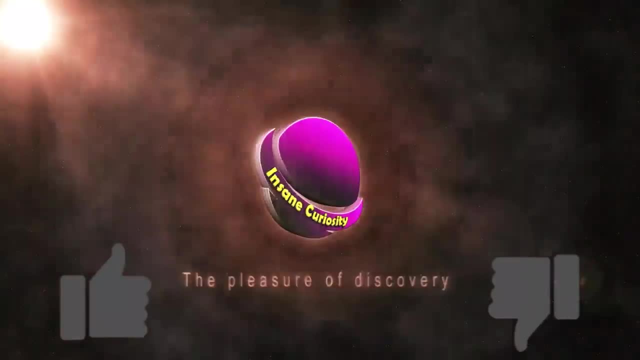 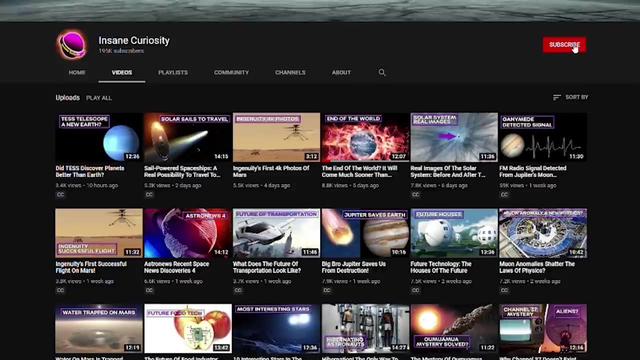 Before finding out what we found about life in our solar system. be sure to like or dislike the video so that we can continue to improve and make these videos better for you, the viewer Plus. be sure to subscribe to the channel by clicking the bell. 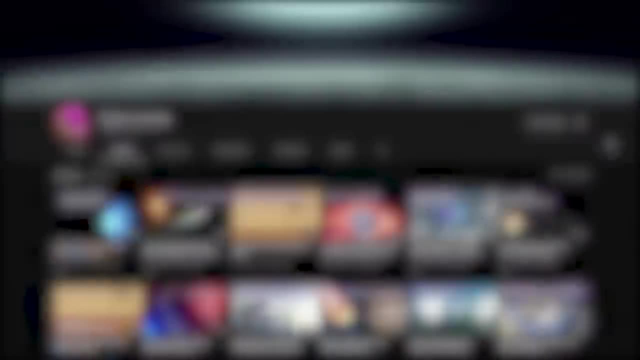 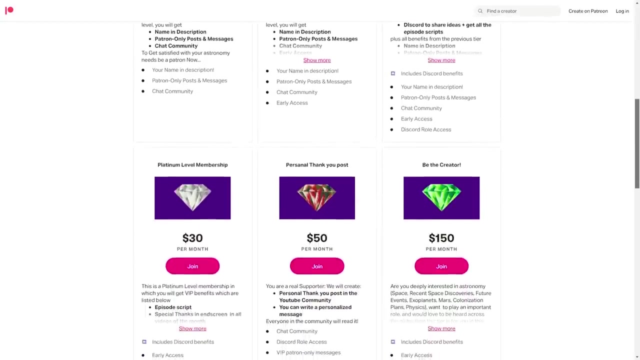 so that you don't miss any of our weekly videos. If you would like to help improve the quality of our content, please check us out on Patreon. we would like to say a big thank you to all those who show their support. EUROPA, JUPITER'S MOVE. 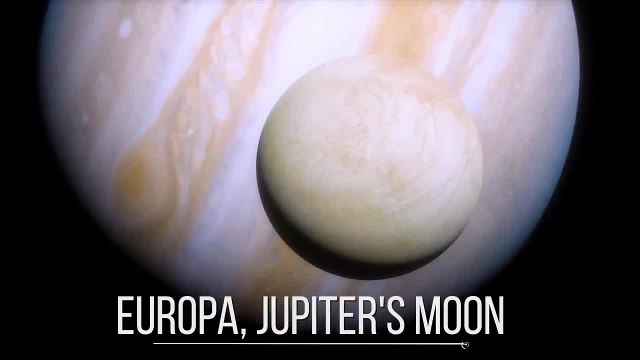 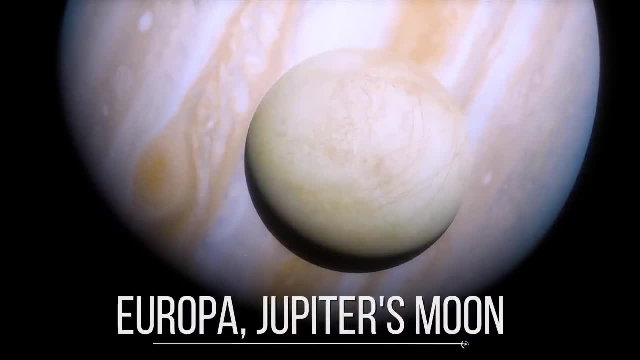 Did you know that the surface of Europa is made of water ice? Many scientists think that beneath the frozen surface is a layer of liquid water, literally an ocean, which is prevented from freezing by the heat from flexing. How do we know it? Evidence for this ocean includes geysers. 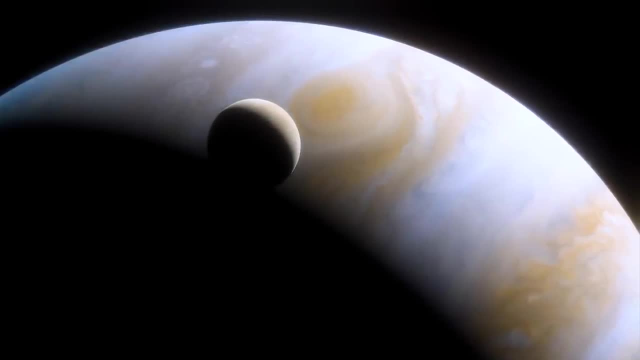 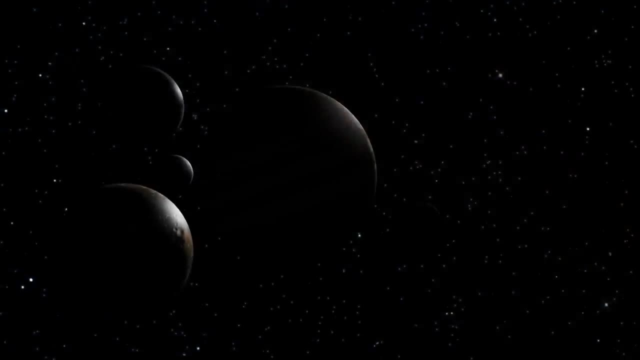 erupting through cracks in the surface ice, a weak magnetic field and chaotic terrain on the surface which could have been deformed by ocean currents swirling beneath, At the bottom of this ocean world. it is conceivable that we might find hydrothermal vents and ocean floor volcanoes On Earth. 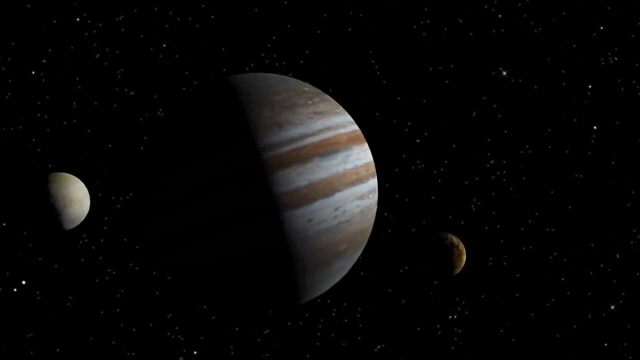 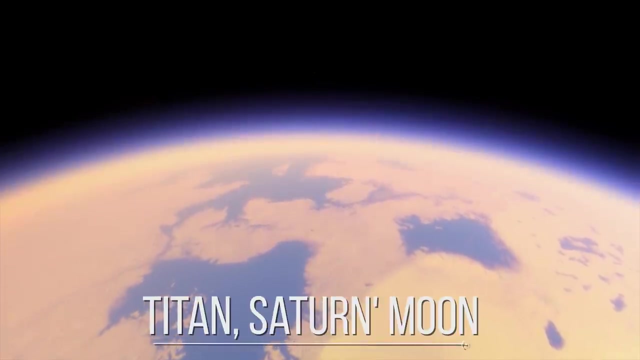 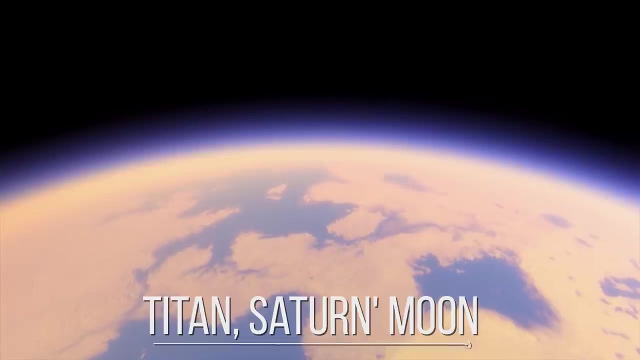 such features often support very rich and diverse ecosystems. Could therefore, Europa host, or have hosted life, TITAN, SATURN'S MOON? Titan is the only moon in the solar system with a substantial atmosphere. The atmosphere consists mostly of nitrogen, which is an important chemical element used in the construction of proteins. in all, 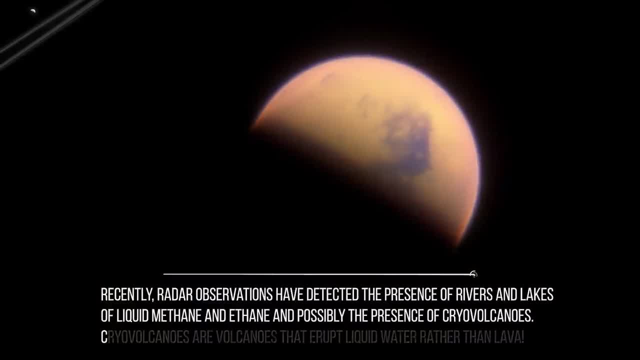 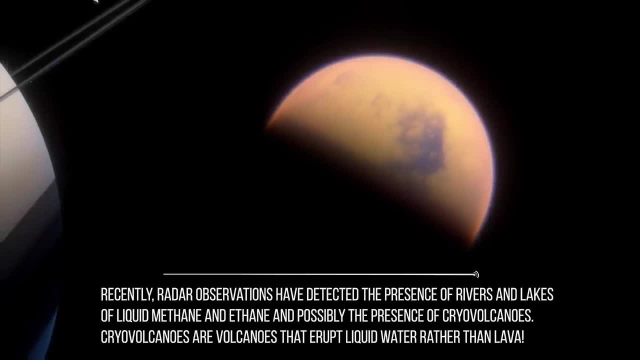 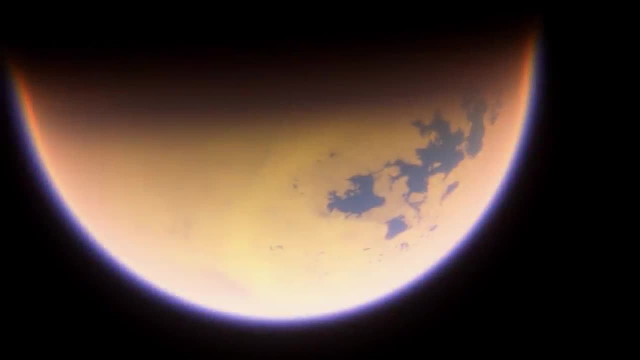 all known forms of life. Recently, radar observations have detected the presence of rivers and lakes of liquid methane and ethane, and possibly the presence of cryovolcanoes. Cryovolcanoes are volcanoes that erupt liquid water rather than lava. This suggests that Titan, like Europa, has a subsurface reserve of liquid water. 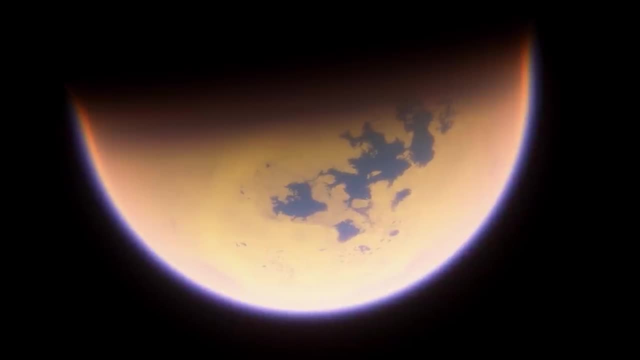 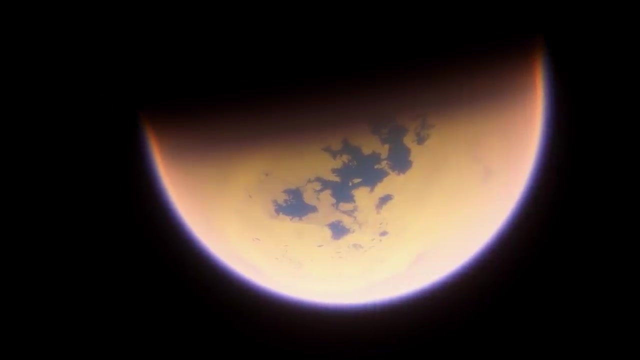 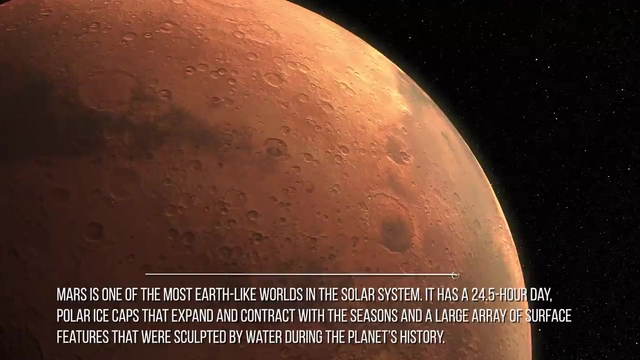 Although it's distant from the Sun, the bountiful chemicals available on Titan have raised speculation that life forms, potentially with fundamentally different chemistry from terrestrial organisms, could exist there. Mars- Mars is one of the most Earth-like worlds in the Solar System. 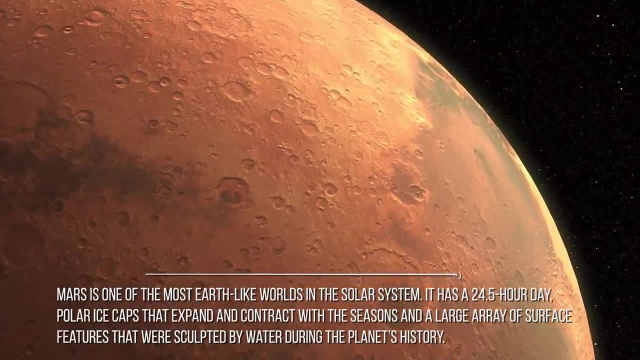 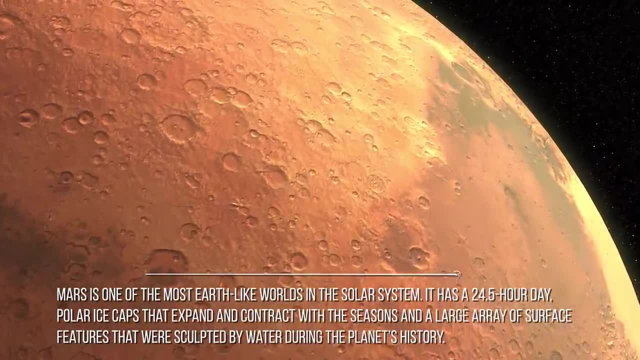 It has a 24.5-hour day, polar ice caps that expand and contract with the seasons, and a large array of surface features that were sculpted by water during the planet's history. Scientists detected the presence of a lake beneath the surface. 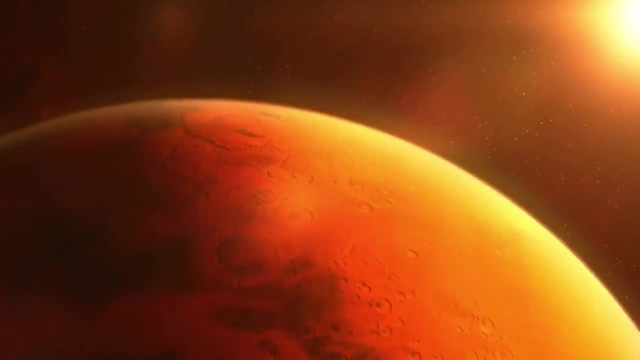 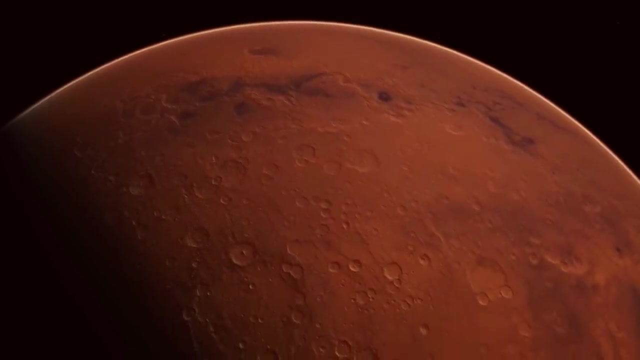 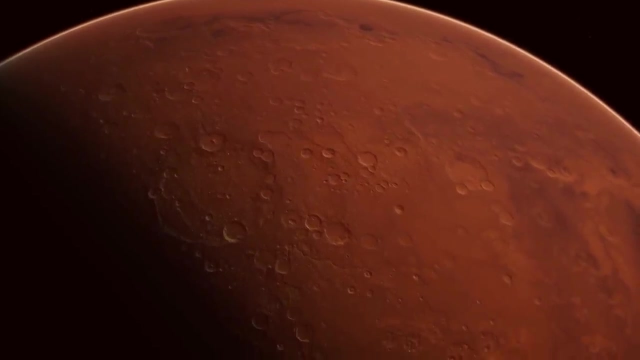 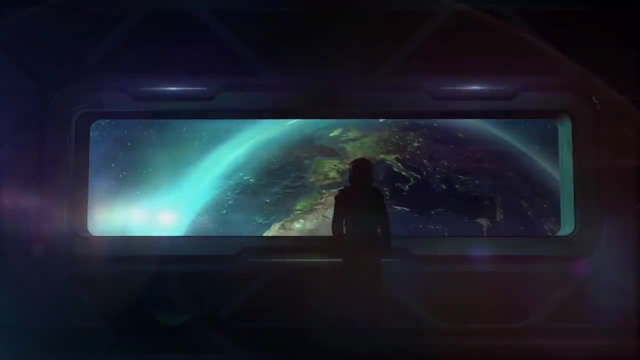 They also found methane. This is amazing because it could be produced by biological processes, even though the actual source for Mars' methane is not yet known. We just have to keep hoping and bringing information from the Martian soil, maybe with the fantastic help of perseverance and ingenuity. 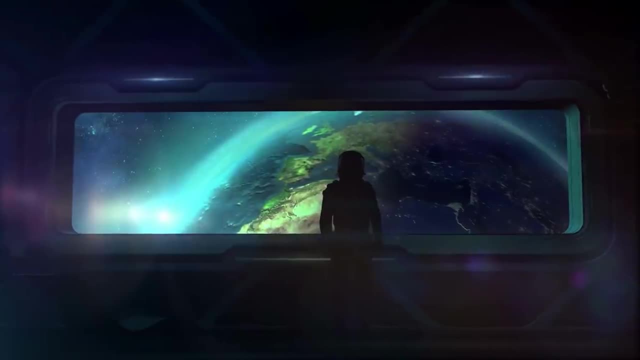 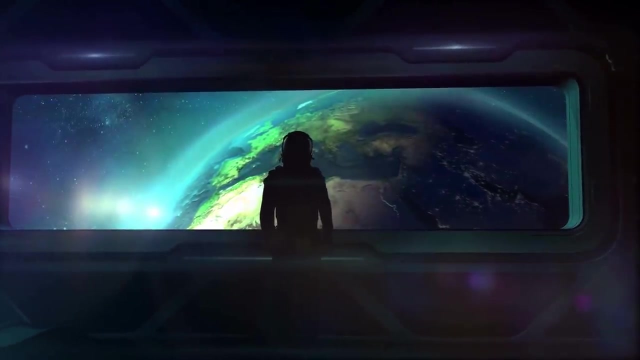 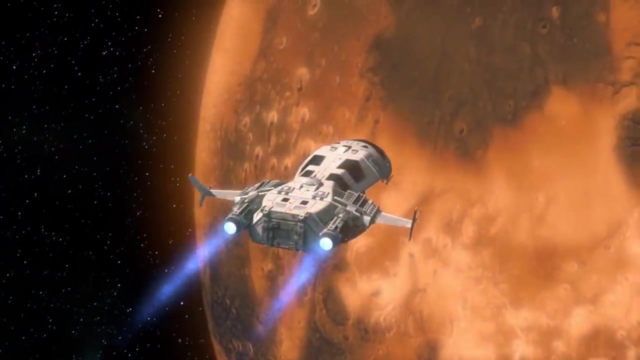 As one can imagine, while astrobiology is a relatively young field, It has a secure and promising future. Astrobiology research has a significant impact on how agencies such as NASA and the European Space Agency plan for current and future space missions. Many recent missions were launched with the aim of exploring worlds in our own Solar System. 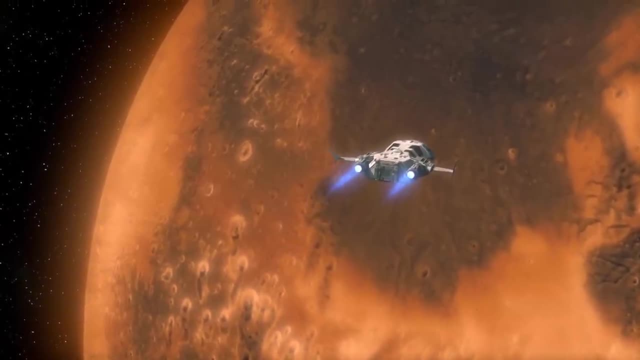 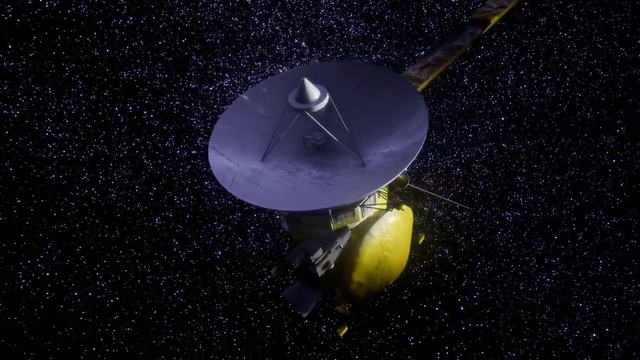 and find signs of past, present or precursors of life, including Mars. One of the most famous missions was the Cassini mission, which gave us a better understanding of Saturn and its moons, such as Titan. Today, we are waiting for the launch of the James Webb Space Telescope, which will allow 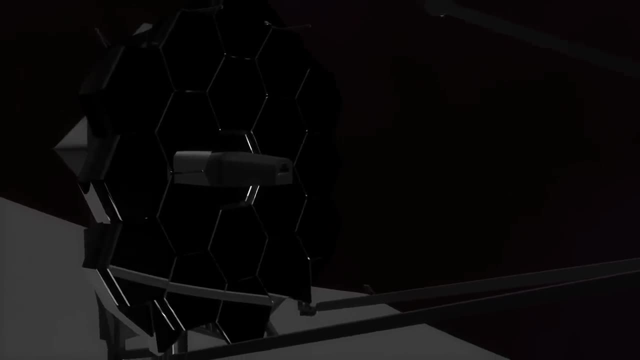 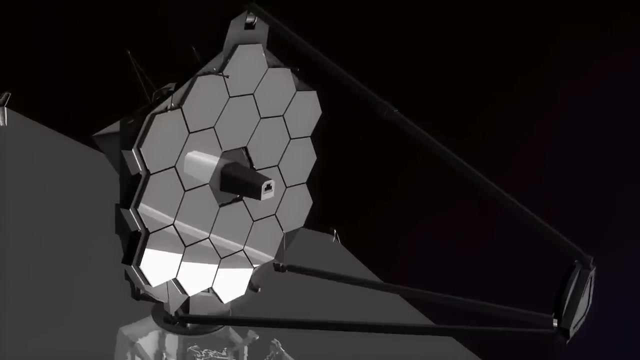 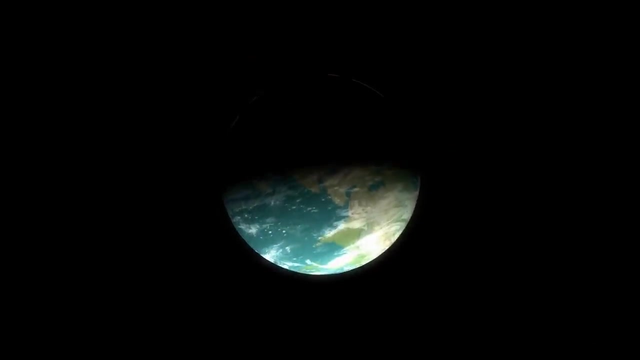 us to begin searching for habitable planets outside our Solar System. Communicating the discoveries and excitement of astrobiology has been understood as a fundamental requirement. since the early development of the field, Meeting this objective has taken various forms. One element was a common form embodied in the Astrobiology Science Conference held biannually.